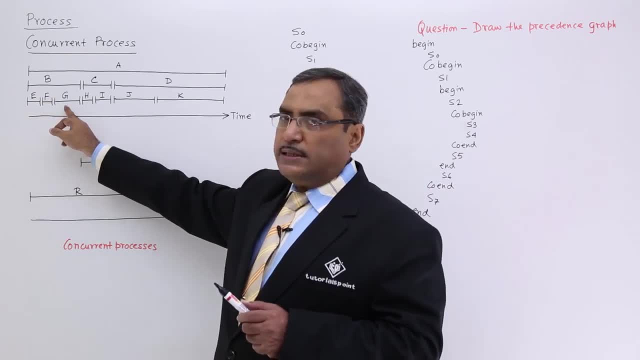 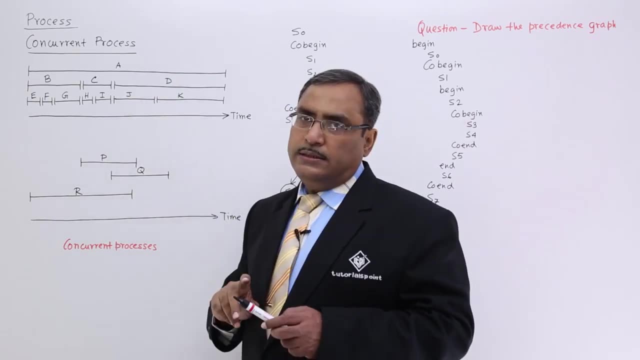 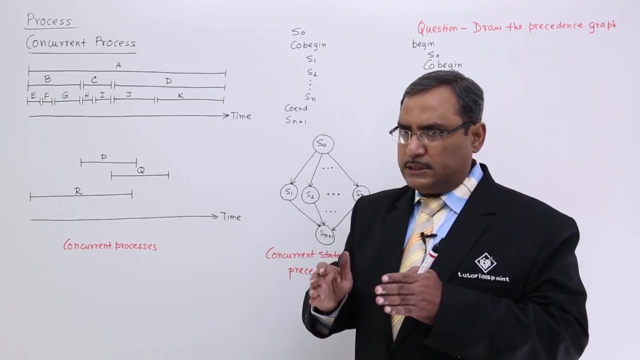 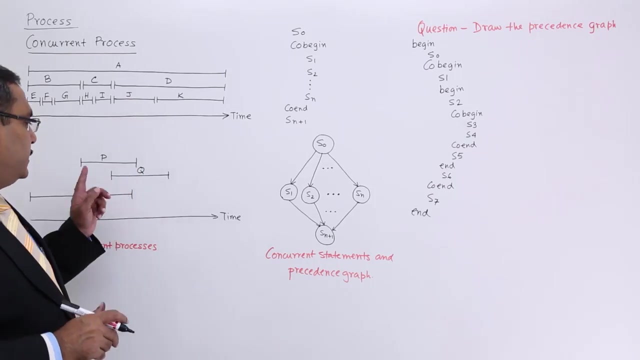 B is consisting of E, F, G sub-tasks, and C is consisting of H and I and D is consisting of G and K sub-tasks in this particular execution. So in this way I can divide a process into multiple sub-tasks or sub-sub-tasks. So simpler operations, sub-tasks, whatever it is. 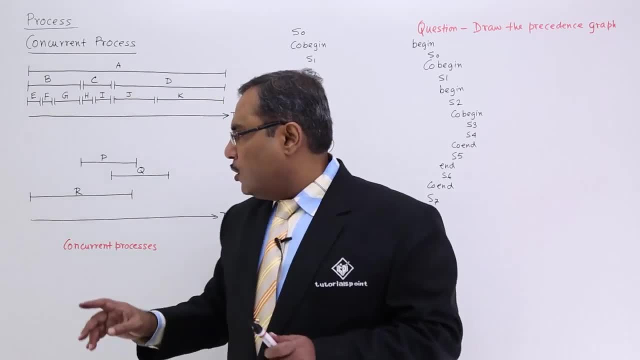 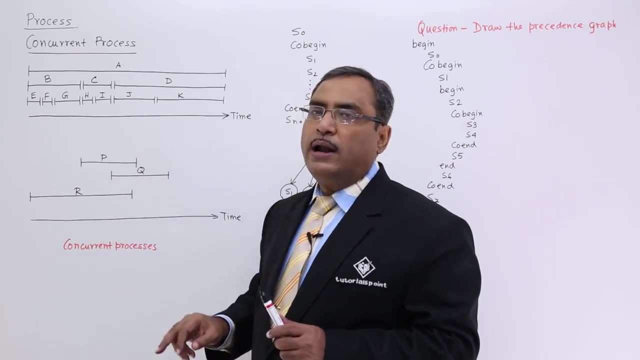 Now let us go for the concurrent process. What is a concurrent process? Concurrent process means P and I. P and Q are concurrent processes. Why? Because they are having some zone where they have overlapped in that execution time span. R, Q, P- all of them are concurrent processes. 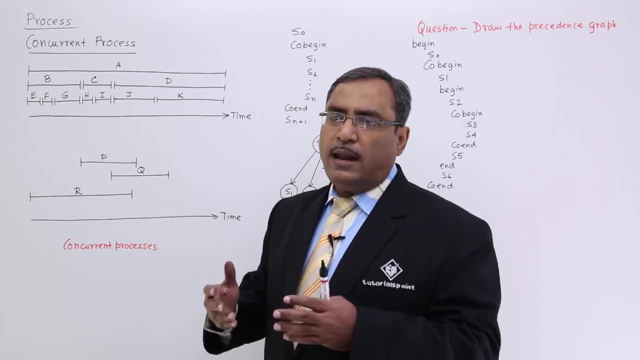 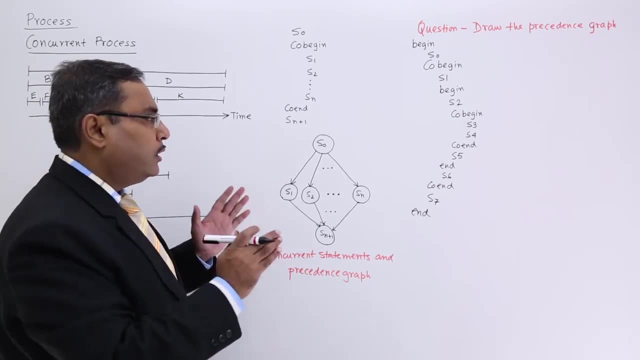 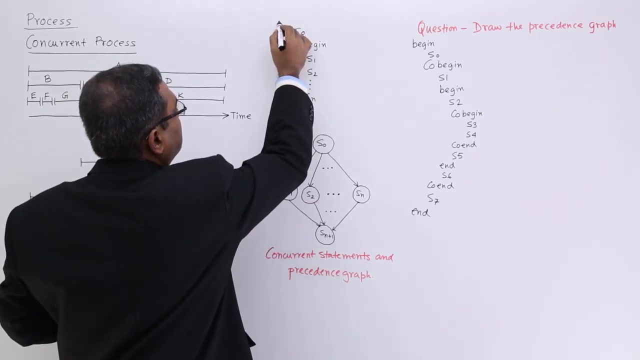 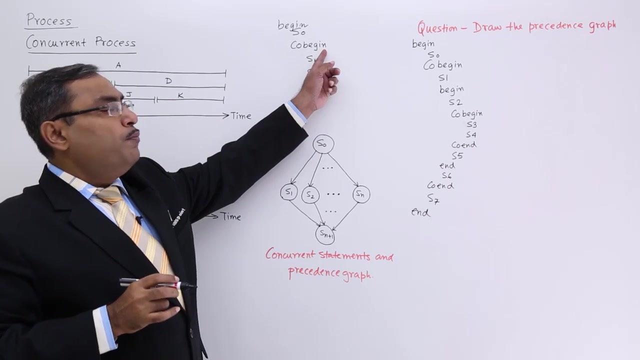 because their executions are overlapping. Good, Now, this is the way to write one concurrent statement or concurrent program code, having the concurrent statements. So I can write this as end. I can put it as begin for the better understanding. So my initial statement is a 0, then co-begin, Co-begin. 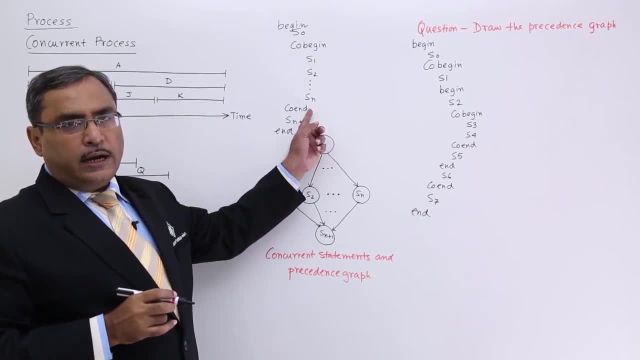 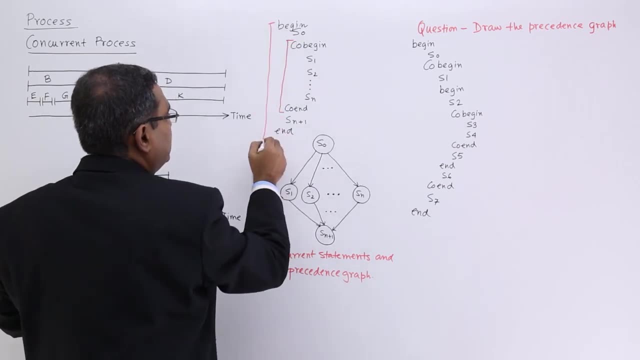 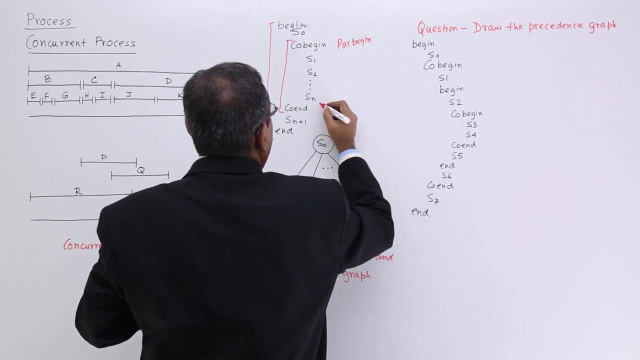 means concurrent begin and co-end means concurrent end. That means that this particular co-begin, co-end, is making one block and this particular begin, end is making another block. This co-begin can also be called as par-begin and this co-end can also be called as par-end, So par-start. 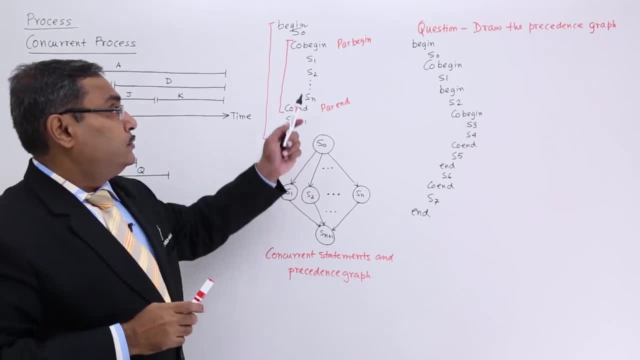 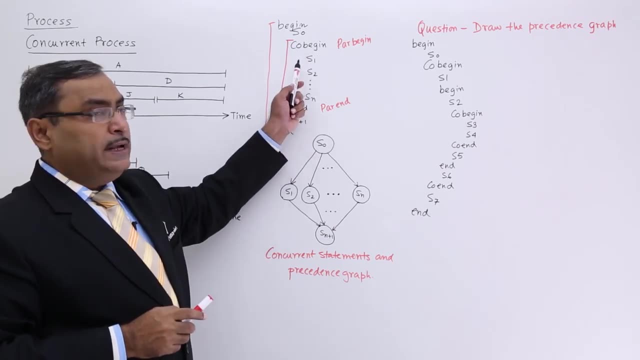 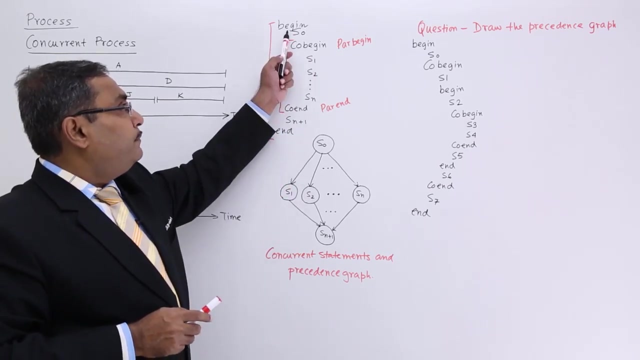 par stands for parallel, Par stands for parallel, So parallel begin and parallel end. So this is the total thing In between co-begin and co-end. I am having statements S1 to Sn and S0, this block and Sn plus 1 in begin and end. So begin and end means all the statements. 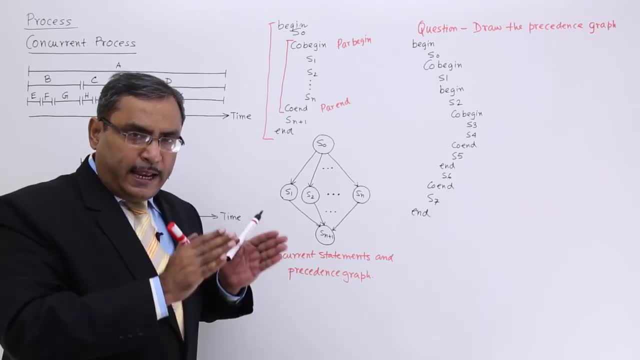 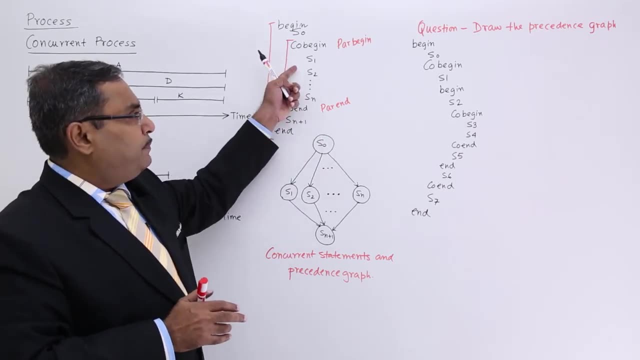 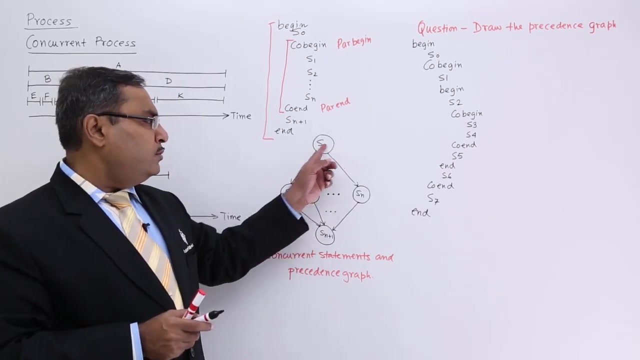 enclosed within begin and end means they will be executed serially, sequentially, but whenever they are enclosed, used within co begin, co end means this statements will be executing in parallel. this is known as the precedence graph. so s 0, this full block, and this s n plus 1 will execute serially. 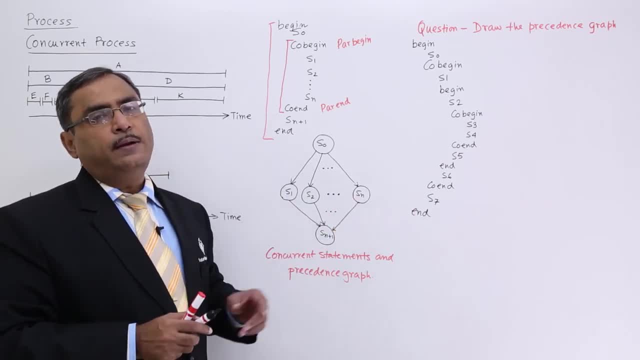 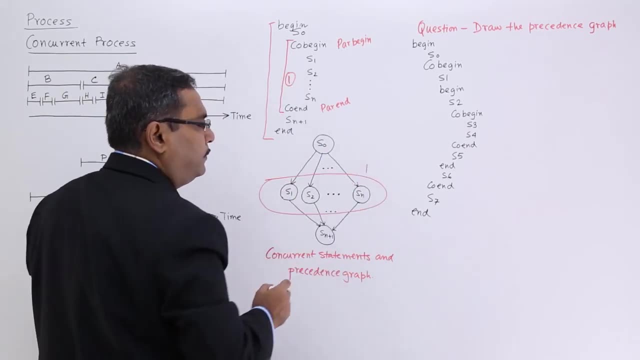 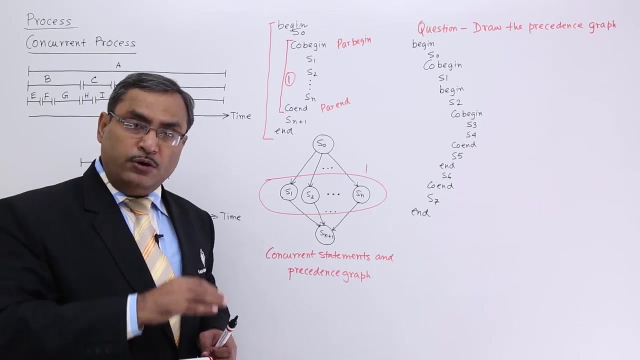 and this s 1 to s n, they will get execute in parallel. so that means, if we mark this particular block as 1, so this is that one block, because they are executing in parallel. so s 0, this block, and s n plus 1, they are executing sequentially one after another because 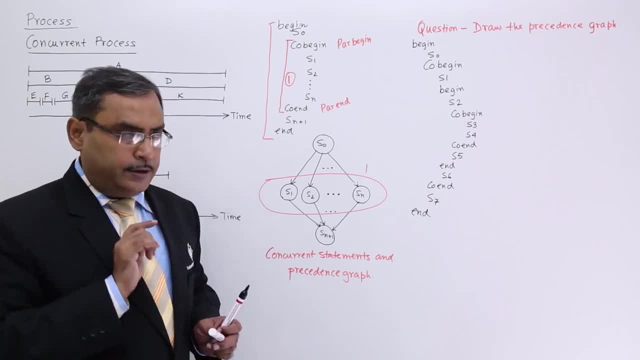 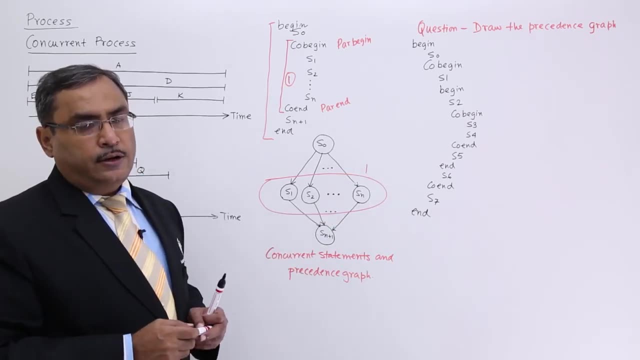 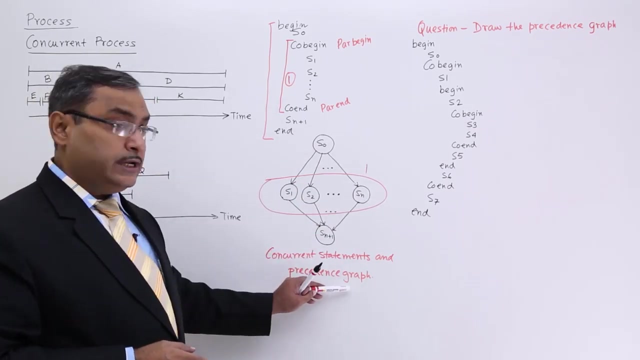 they are enclosed within begin and end. question: draw the precedence graph for this following code. so that is a question: draw the precedence graph for this following code: so this graph is known as precedence graph. i have mentioned that one here, so let me answer this particular query. ok, now we are having 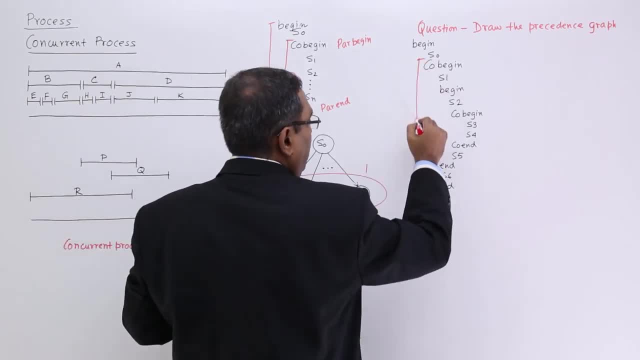 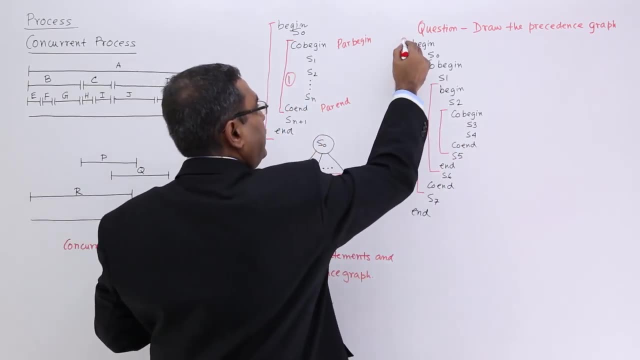 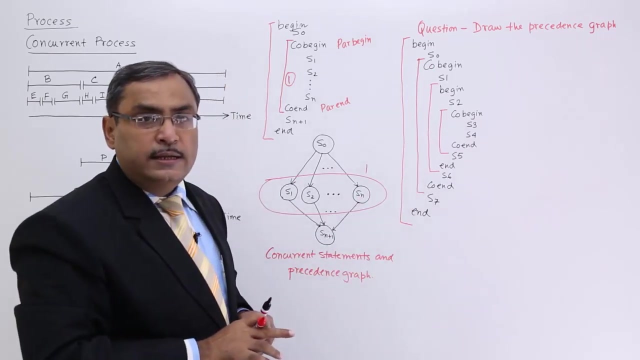 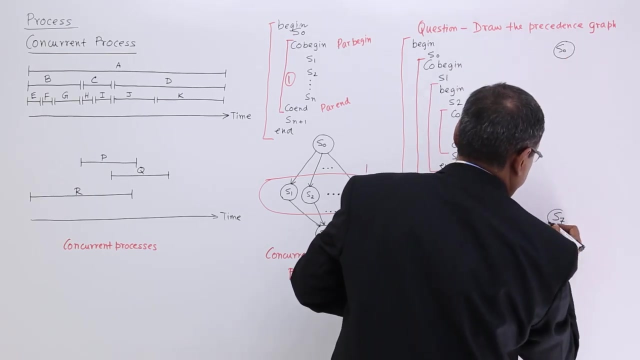 s 0. so let me do the marking of the blocks. so they are coming like this and that is the begin end. this is the outer block, so s 0 and s 7, and this block will be in series. so let me write. so: s 0 will be at the top, s 7 will be at the bottom and this very block will. 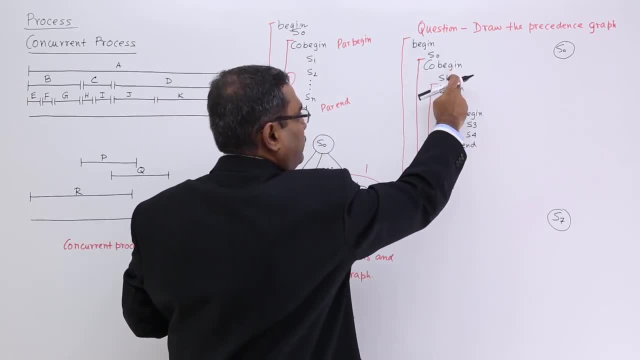 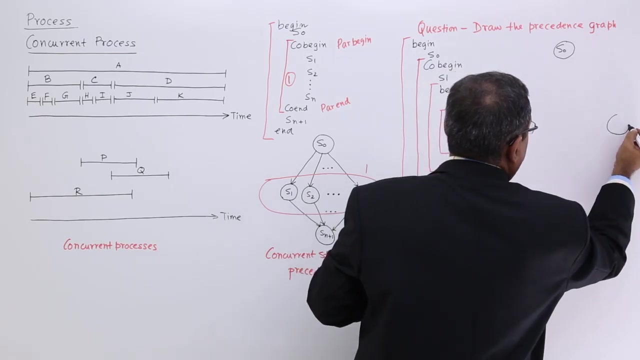 be under this: b, s 1, b, s 1, b c, S 1- this block and S 6 in parallel, because they are in co-begin co-end. So S 1, this block and S 6.. So I shall be having S 1 here. some block will be there then I shall be. 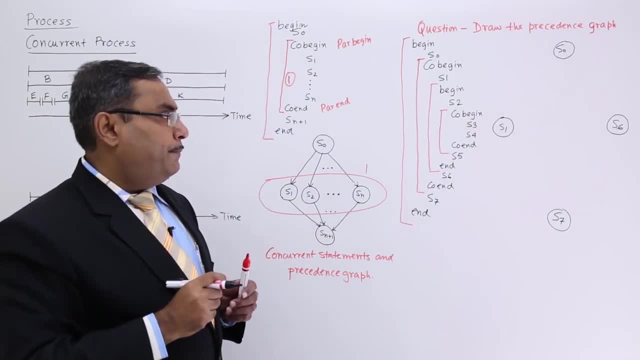 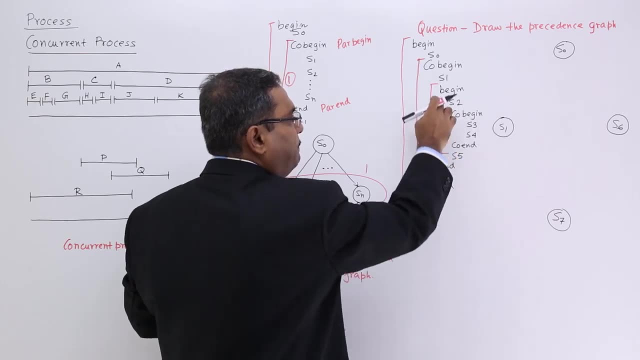 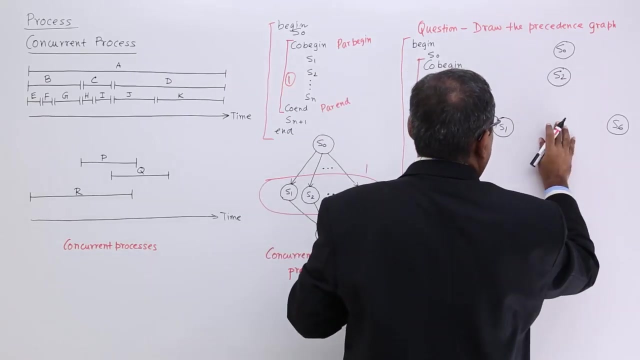 having S 6.. Now, what about this block? This block is having S 2, some block and S 5, and they will be under begin end. that means they will be serial. So I shall go for S 2, something. 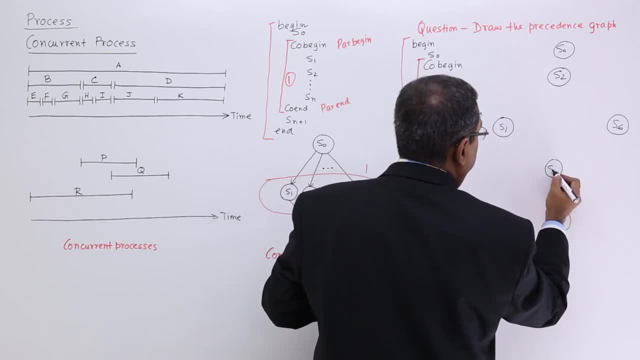 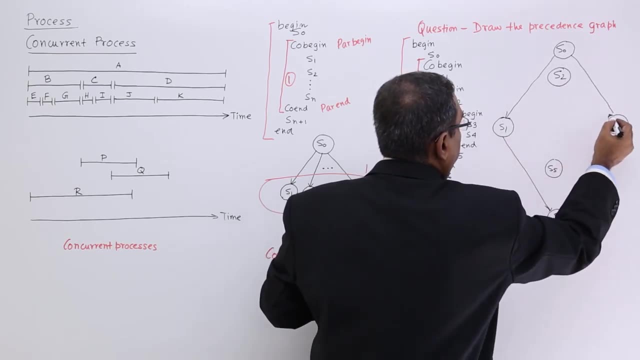 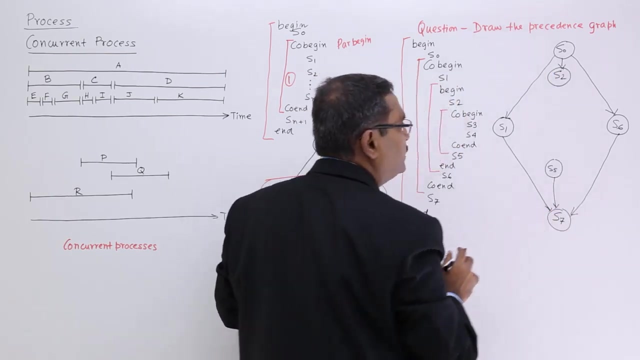 will take place, and then here I am, getting S 5. So it will be coming like this, it will be going like this, it will be coming like this, and then it will be coming like this. So this much, we have done this much. 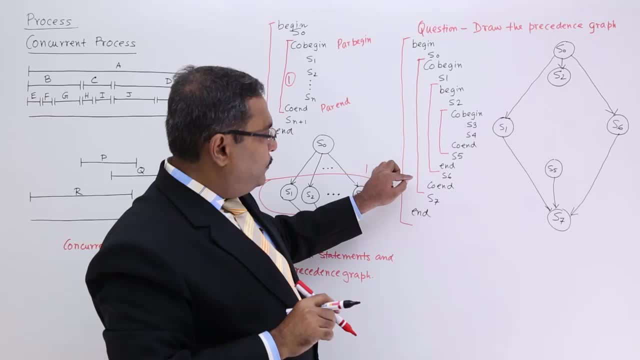 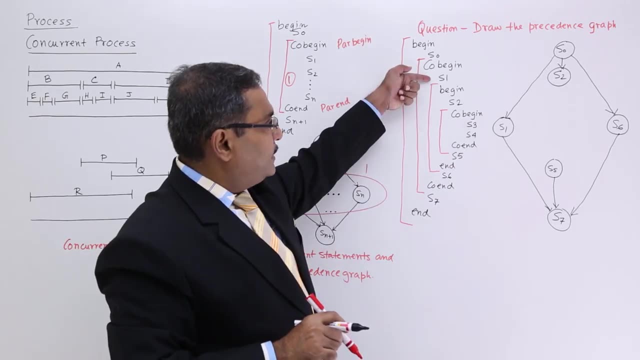 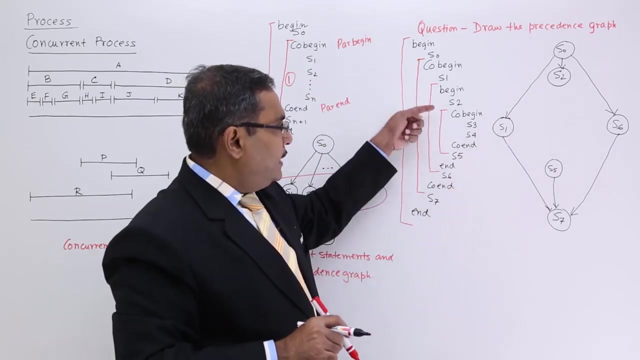 Again, you see S 1.. Sorry, S 0- this block, and S 7.. So S 0, this block and S 7.. Now, in between co-begin co-end: S 1- this block and S 6.. So S 1, this block and S 6.. Now here, in this case, S 2, S 5,.